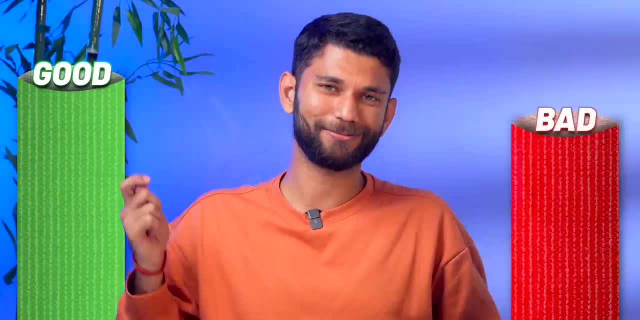 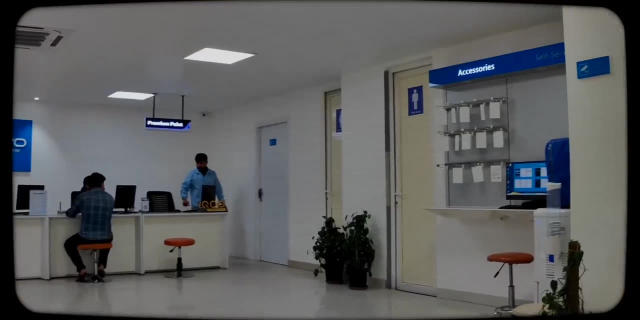 iPhone 15 Pro Max- best camera in a phone- good, But it costs 1.6 lakhs- bad. We tried 100 plus smartphones this year, 2023.. Visited service center for every single brand. So which brand is good for you in 2023? 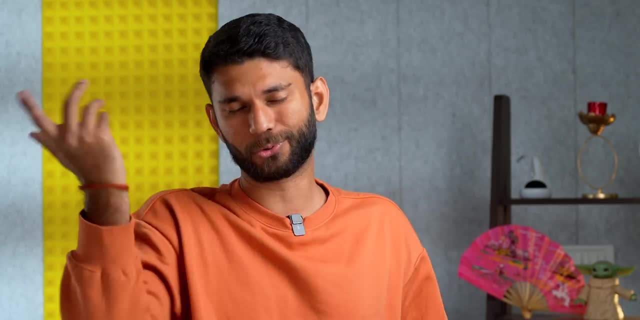 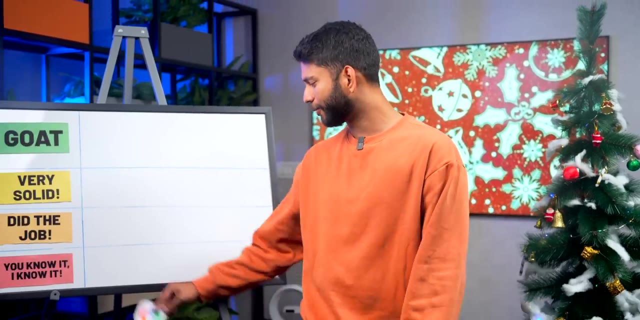 and which are the brands that need serious improvement and you should definitely avoid. obviously, Now, to make things easy and simple for you guys, we'll be ranking the smartphone brands in tier. We'll start from the bottom and slowly move to the best brand in 2023.. 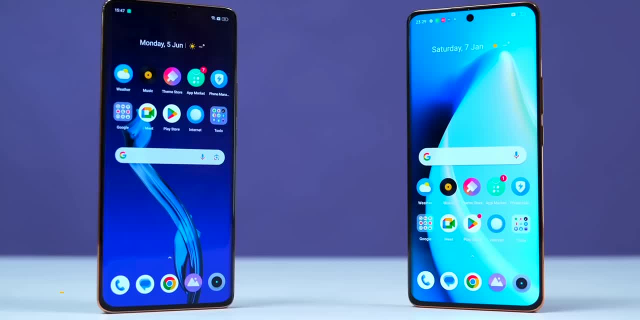 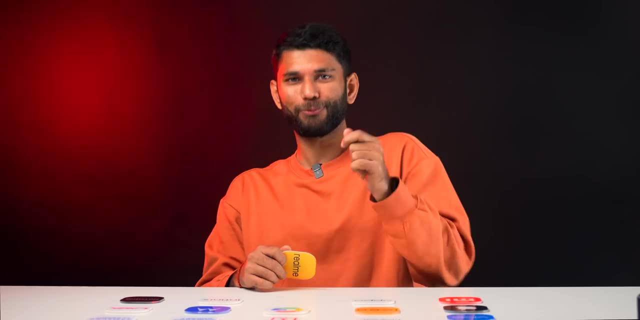 Okay, first up we have Realme. They launched very few smartphones this year. The most popular Realme 11 series was like: okay at best. I mean it is absolutely fine to launch few phones, but then at least make the phone so good. 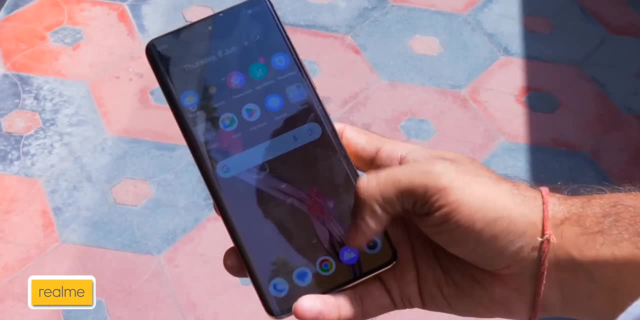 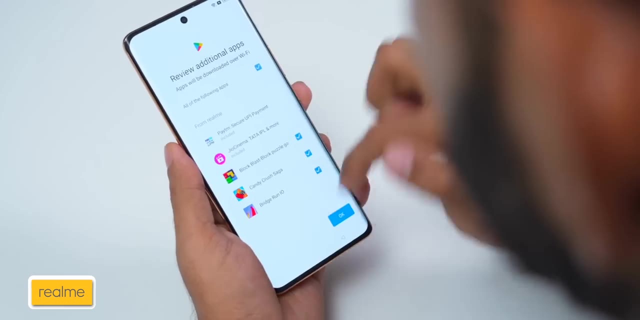 that other people take notice. That was in the case here. Realme 11 was very mediocre: Average camera, Passable performance and all of that. But what got worse this year is the software experience, Because Realme OS was filled with bloatware and inappropriate ads. 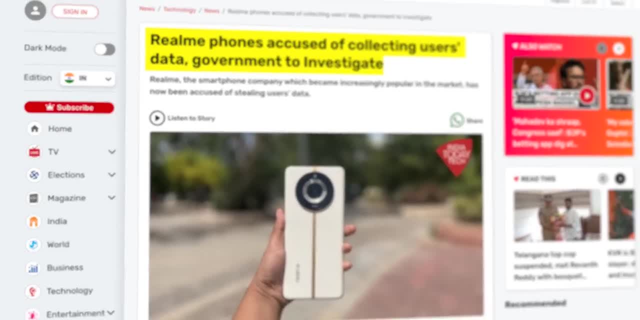 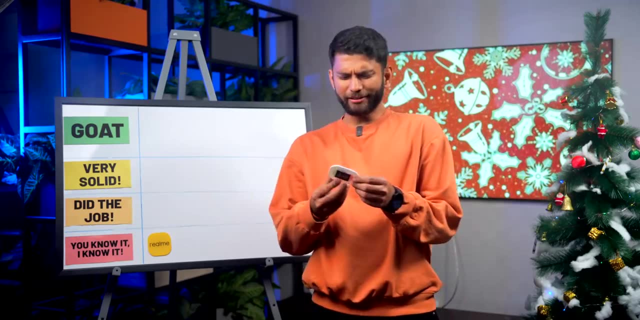 Then there was the whole data collection controversy, where even the Indian government had to inquire about Realme. So I'll put Realme in the- you know it, I know it- tier. Another brand that kind of disappointed me this year is Google. Now, I know I'm going to get a lot of flak for this. 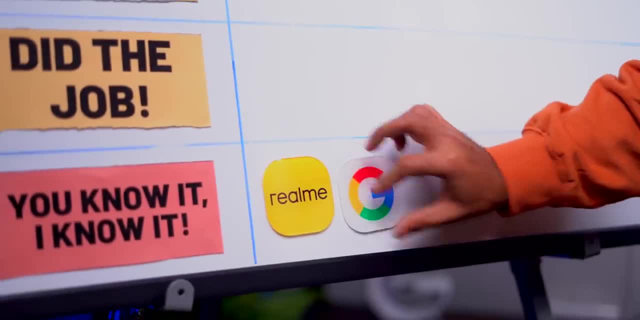 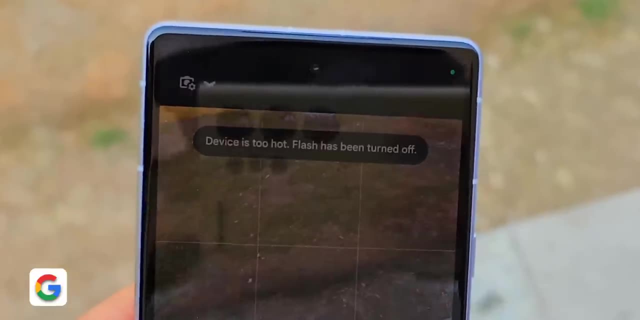 but I'll put Google in the. you know it, I know it tier. Well, hear me out. So Google launched three phones in India in 2023.. All of them had similar issues: They get hot performance, for the price is average. 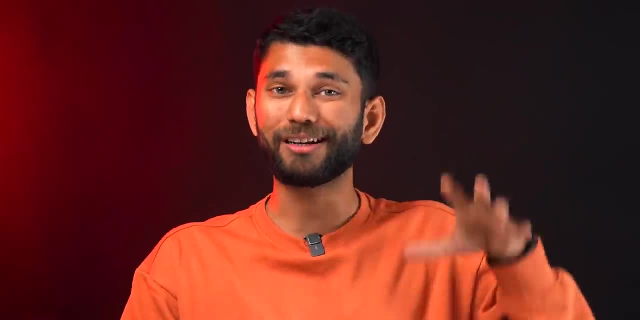 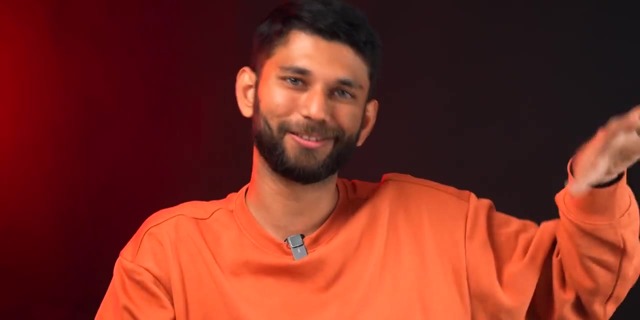 and most of the AI software features that Google promised have started arriving now or will come in 2024.. But you buy a phone for what it is right now and not for what you get promised in the future. I'll leave all of that aside. 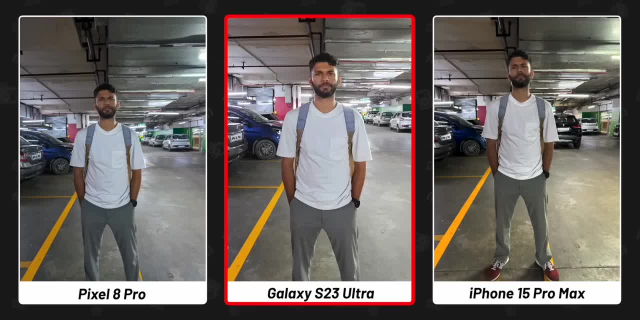 Let's talk about the camera. Like the Pixel, phones are known to be the camera king, but we have used the 8 and the 8 Pro extensively and side by side with the competition. the photos from the Pixel 8 series were just average. I just hope that the Pixel 8 series will come out in the near future. 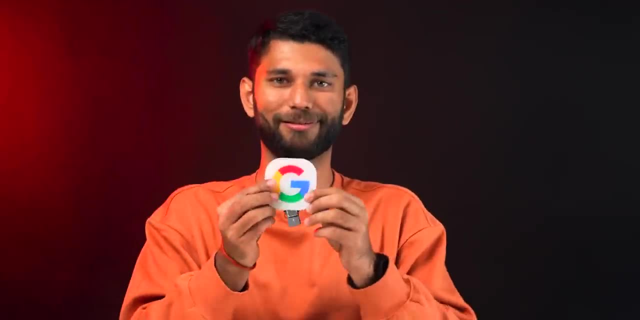 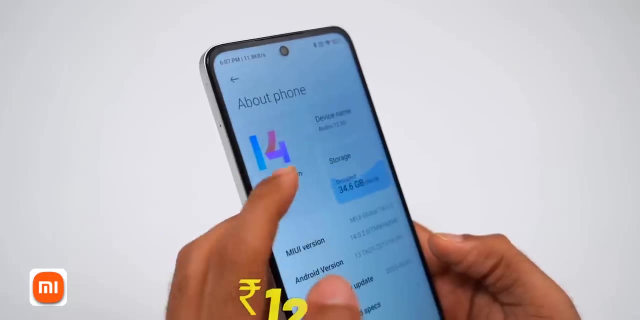 I hope they bounce back to full potential in 2024. and Google, please, please, fix your Indian pricing, please. Moving to Xiaomi, we have the Redmi and Poco phones. The base Redmi 12 was a good phone. It launched for around 12,000 rupees. 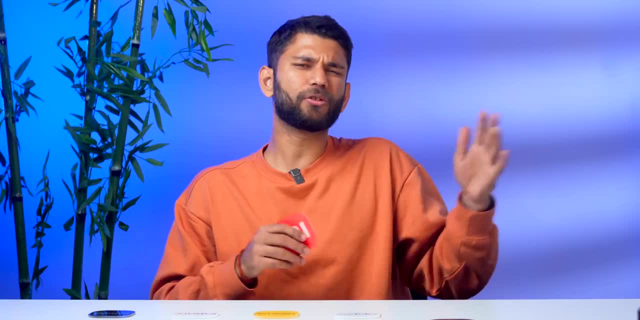 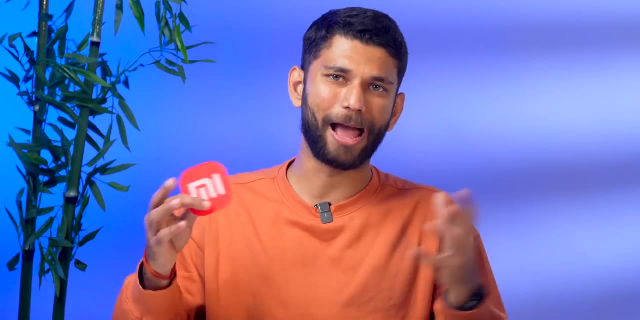 and it is a 5G phone with glass back and all of that. But the rest of the series was average at best, Like the phone launched with Android 12. that is like a year old software. And then there was the whole Poco and motherboard fiasco. 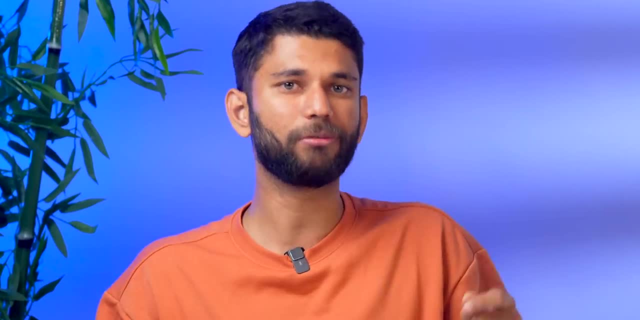 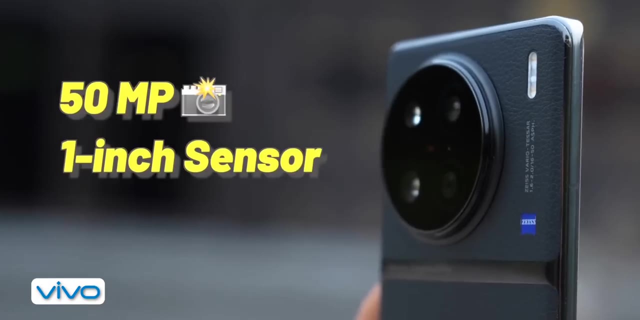 We have covered that extensively in this video. You can go check out if you want to after watching this video. So I'll put Xiaomi in. did the job tier. And then we have Vivo. The Vivo X series were great camera phones, like some of the best photos we have taken. 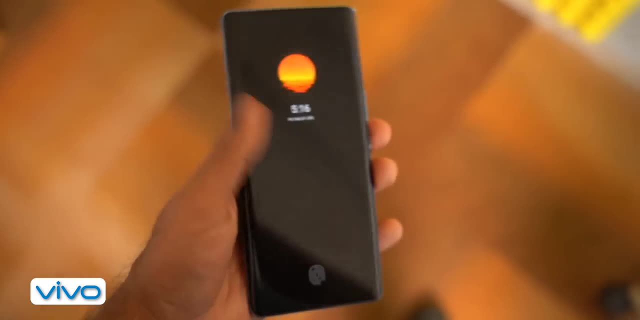 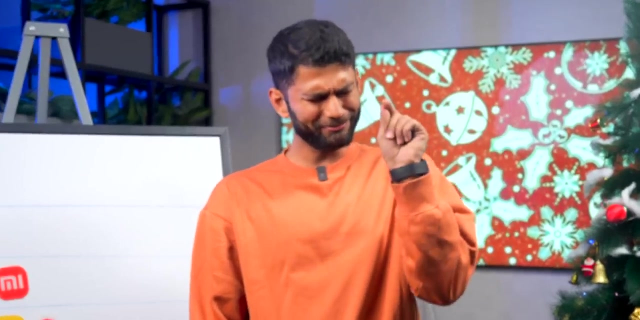 But overall the Vivo portfolio was okayish, Like there is Vivo V series. V27 was a good launch But by the end of the year we got Vivo V29, which was the same as Vivo V27, with some extra itsy bitsy features here and there. 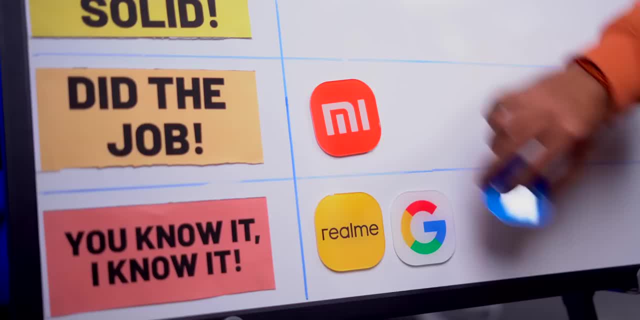 Vivo in 2023 did what was expected of them to do, So we'll put Vivo in. did the job tier. Coming to Oppo: well, this was kind of fun. Oppo launched their flip phones for the first time in India. 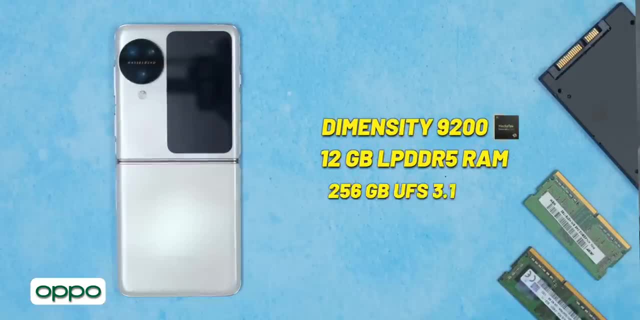 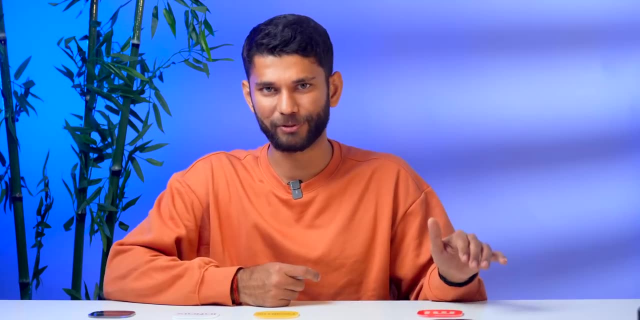 The Find N3. And the hardware of the phone was good. Vertical cover screen was great for watching shots and reels. Even the camera was nice. However, the software experience was below average. Plus Oppo completely messed up with the pricing, Like the Oppo Flip launched for 95,000 rupees. 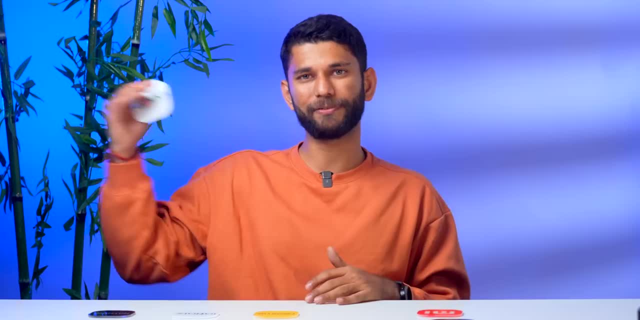 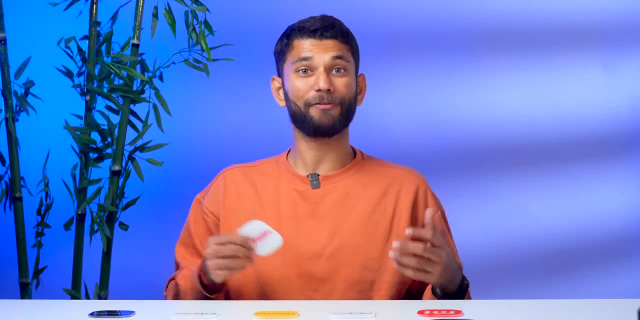 In a world where the Samsung Flip already exists for 95,000, Oppo Flip wasn't really a good choice. So Oppo goes into the did the job tier. Next up, we have upcoming brands And I must say this was unexpected. 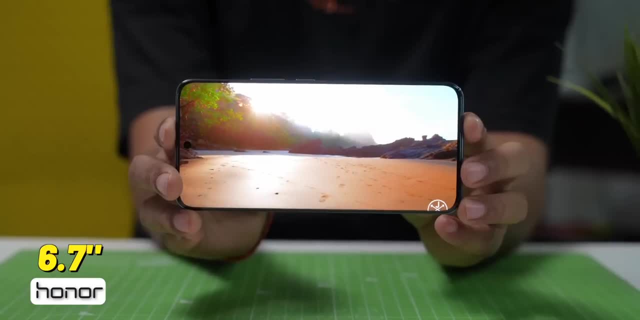 Take Honor, for instance. In 2023, they sort of made a comeback with the Honor 90. It has good specs, decent camera and overall, a well-rounded phone. Only thing was it was priced for 35,000 rupees. 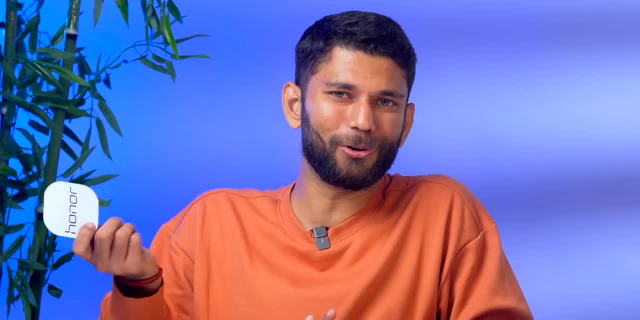 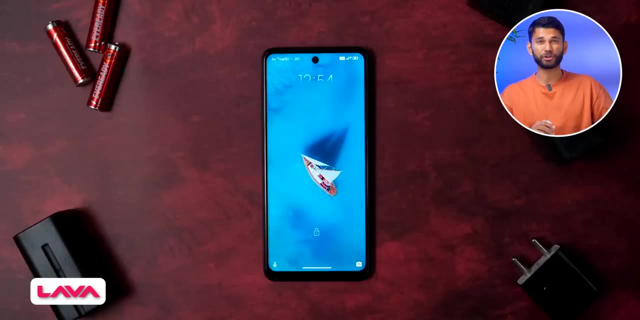 Then the price was reduced back again, So Honor had to do more launches to have an opinion on it. So it goes in the did the job tier. Then there is Lava Blaze 2 was a good 5G phone under 10,000.. 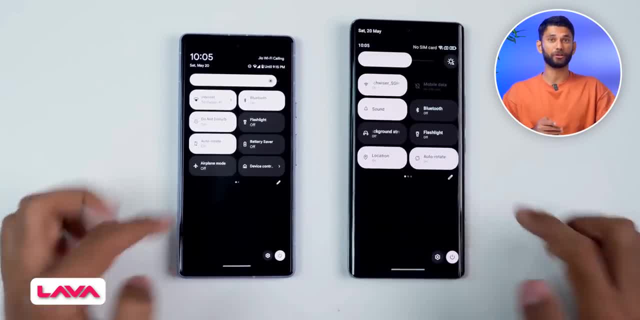 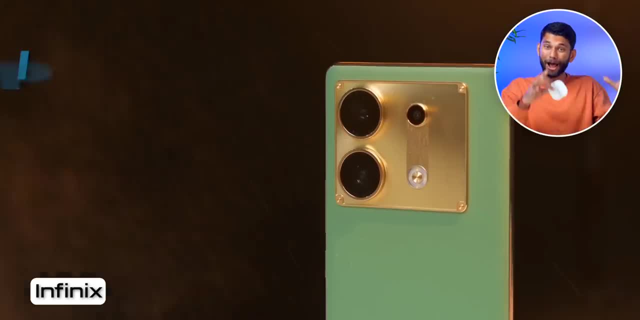 And the Agni 2 was a good phone with stock Android under 20,000.. And then there was Infinix. They had pretty great launches with the Zero 35G, which had 4K selfie video, OIS, and all of that for around 20,000 rupees. 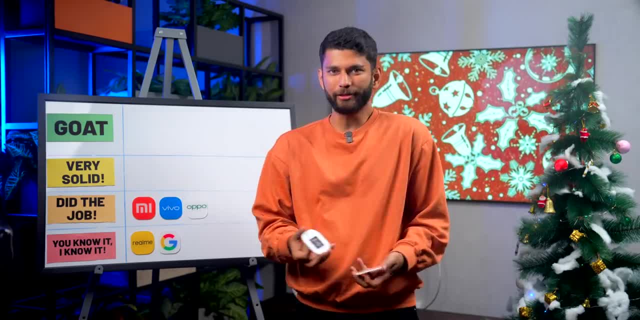 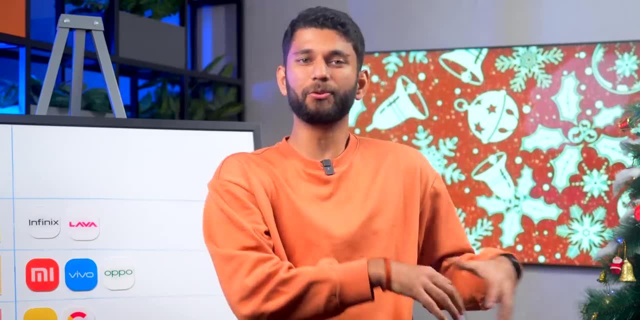 Like. both of these companies launched really good phones in their price segment, So I'll put both of them in very solid tier And I'm very hopeful of all these upcoming brands. If they stay the course, they could seriously give other brands like Xiaomi, Realme a run for their money. 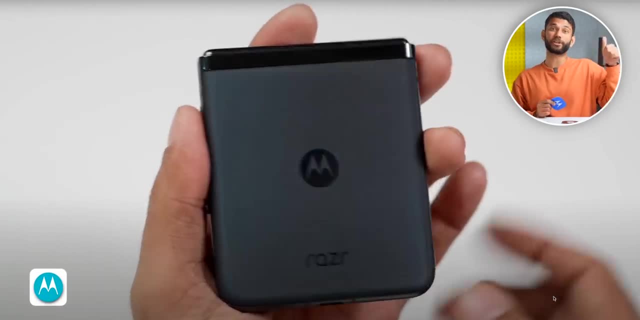 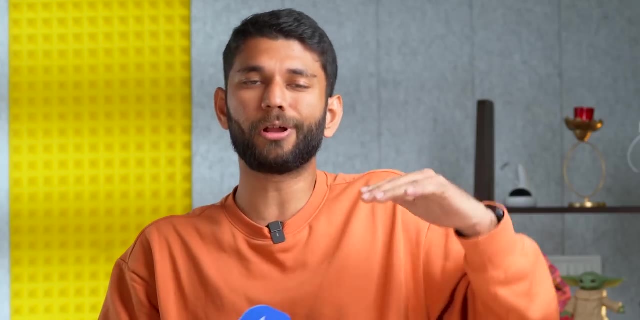 Speaking of Motorola, they launched some really nice phones this year: Moto Razr 40 Ultra, first flip with a big functional cover screen, And the Moto Razr 40,, the most affordable flip in the market. And not just this: Motorola brought flagship features on budget. 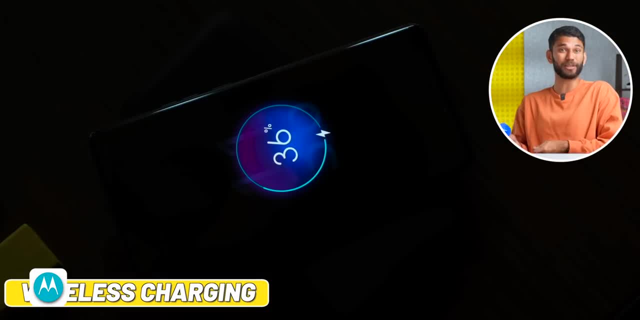 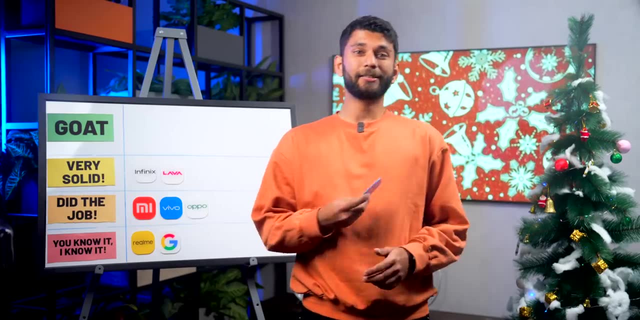 Curved display, 144Hz refresh rate, wireless and reverse, wireless charging, IP rating. all of them- Edge 40 and Edge 40 Neo- were one of the best phones in their price. That being said, there are still two things that Motorola needs to look into. 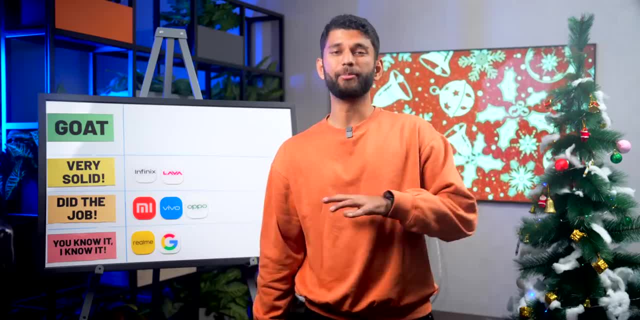 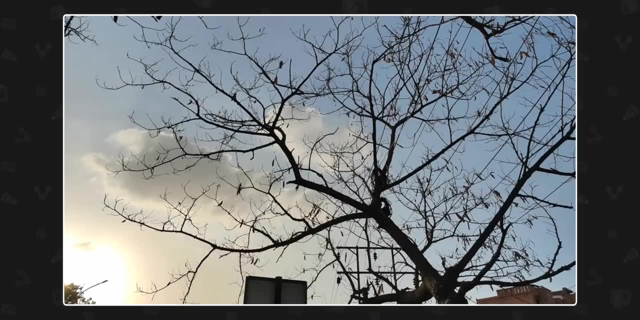 First software update, Like it got better than 2022, but it is still behind other companies. And second camera performance, Be it in budget, mid-range or the premium flip category, Motorola's picture were at best average or slightly below average. 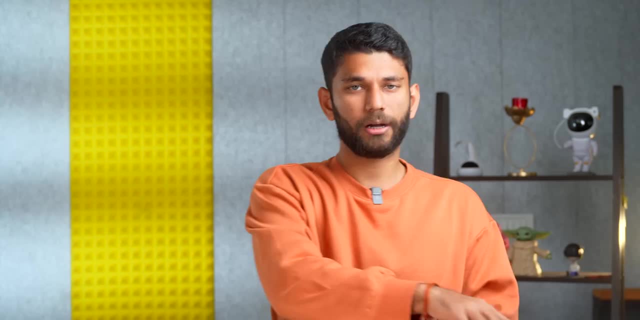 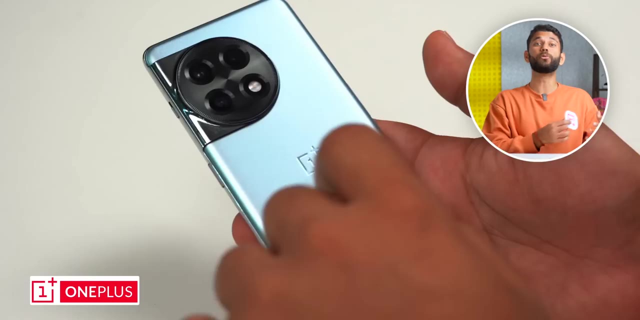 So I'll put Motorola in the very solid tier. Another brand that goes in the very solid tier is OnePlus. 2023 was a comeback year for OnePlus. OnePlus 11 and OnePlus 11R were really good phones for the price Plus. they launched their first foldable phone, OnePlus Open. 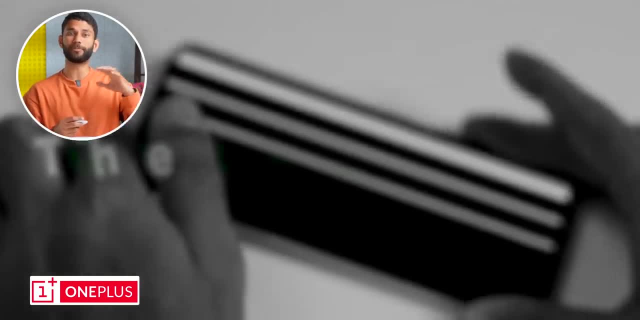 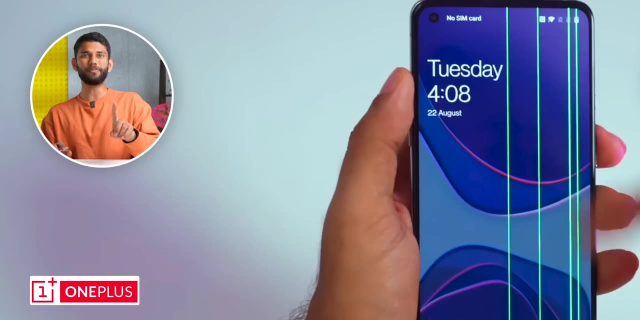 which was kind of an unexpected hit. Another thing worth mentioning: while many brands got this green line of death issue on their phones, even older OnePlus phones were affected. OnePlus was the only brand to announce three replacements, even if the phone were not in warranty. 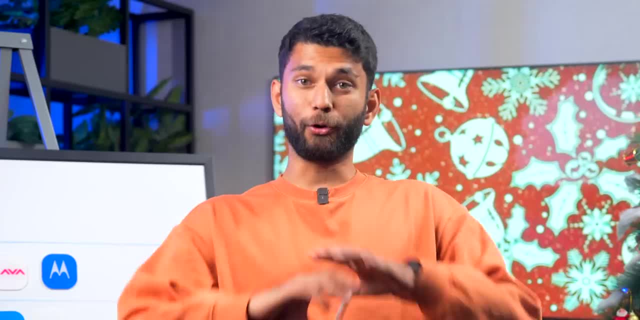 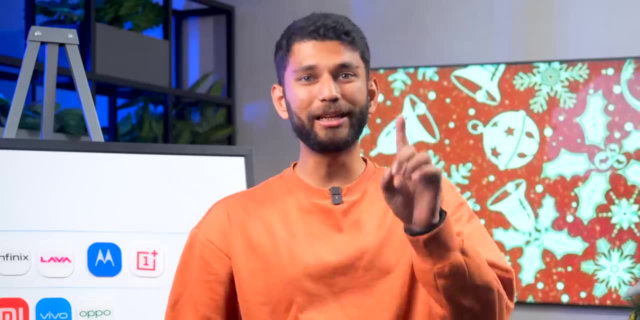 So it was bold and good from OnePlus to announce this publicly. For all of this, OnePlus finally goes to the very solid tier Because, while most of it was good, OnePlus was the only brand to announce three replacements. The one area where OnePlus really struggled was in camera. 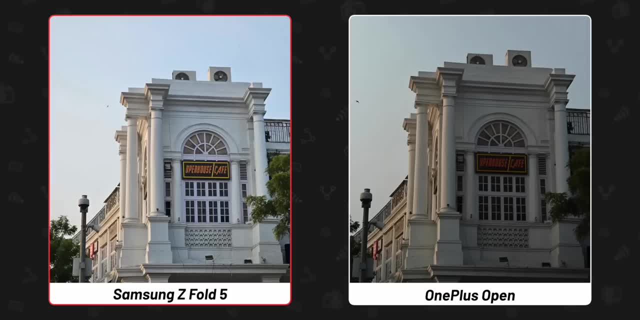 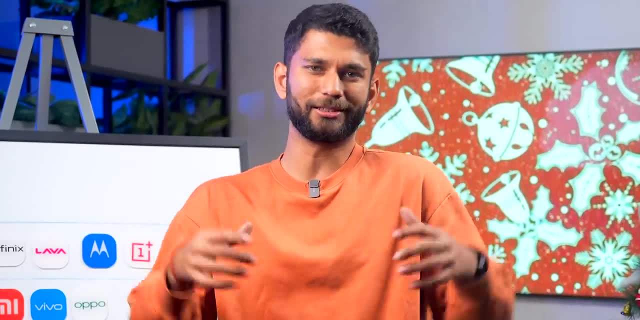 Be it OnePlus 11, 11R or even the OnePlus Open. if you compare the camera with other phones in that same price range, OnePlus kind of fell short. But very solid is very solid. I just hope they double down this in 2024.. 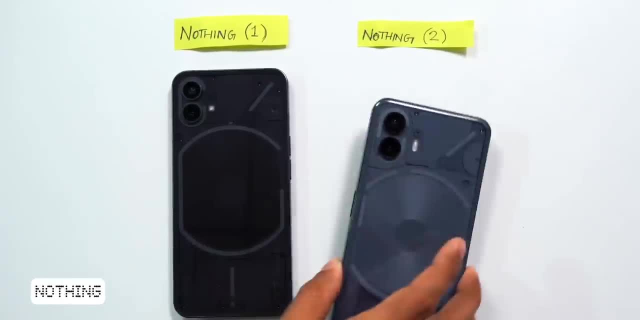 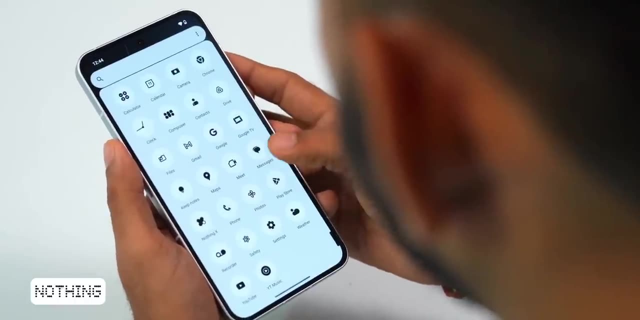 Another end trend in the very solid tier would be nothing. Phone 2 was a good phone. The Glyph interface is still unique and brownie points for the excellent software. Also, they recently released their Nothing OS 2.5,, which is based on latest Android 14.. 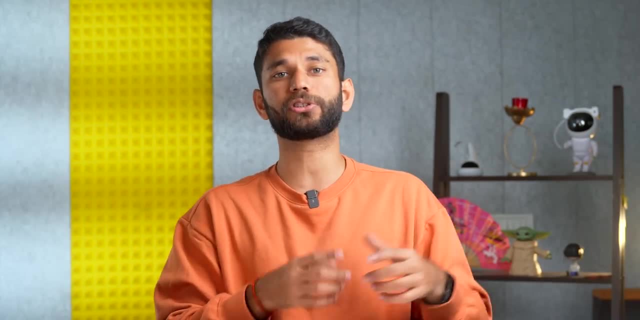 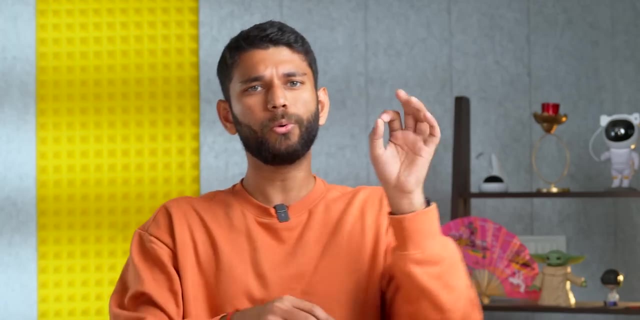 This is faster than many other smartphone brands. The company also launched a sub-brand, CMF. We got this TWS for ₹2,500 and this smartwatch for ₹4,000.. Both of these were really good for the price. Now, the only thing with Nothing was their weird pricing strategy. 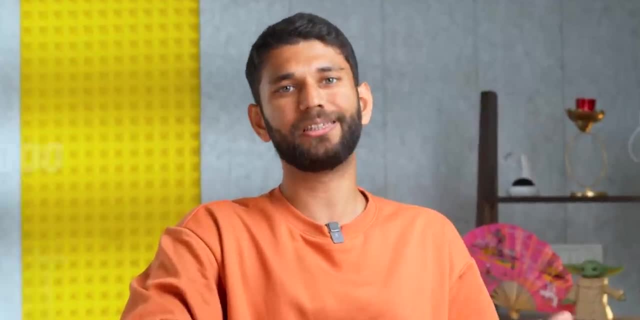 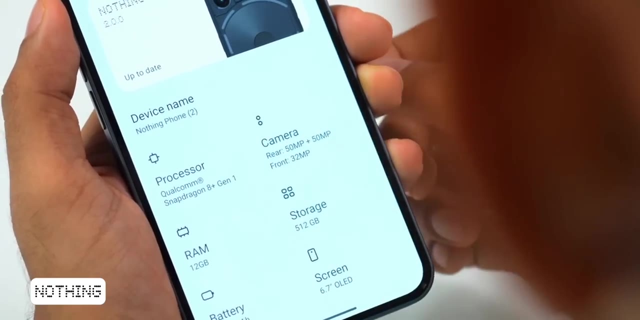 Like the Ear 2, launched for ₹10,000 in India. For reference, the Ear 1 from the previous year came for ₹6,000.. Same for the Nothing Phone 2.. 8 Plus 1 Gen phones from other brands launched for ₹40,000,. 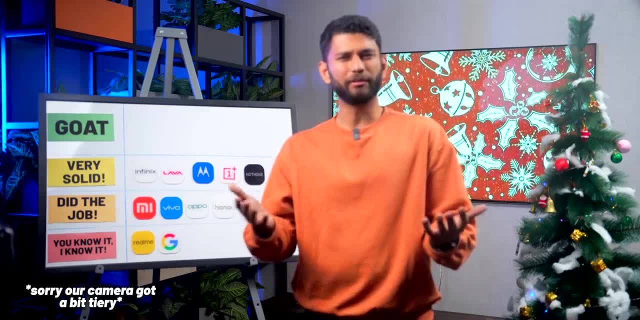 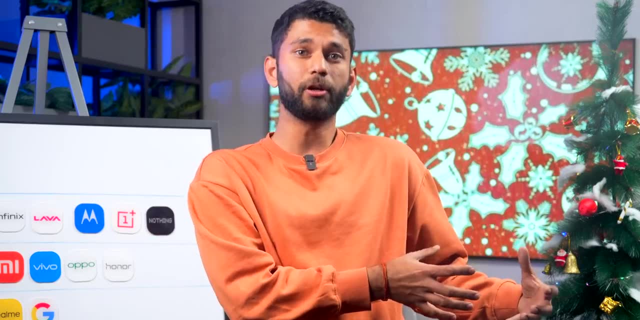 but the Phone 2 launched for like ₹45,000. So price was something they had to still nail in India. So yeah, not good but very solid. I hope Nothing takes note and improves the price. The pricing strategy in India in 2024.. 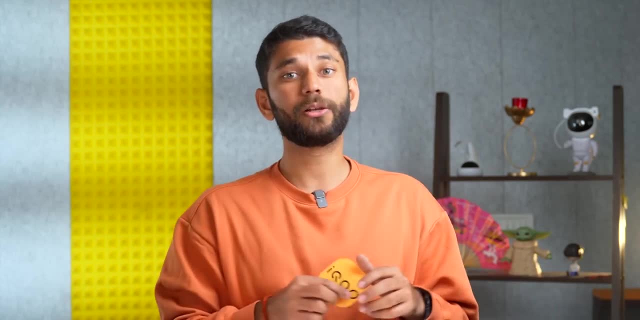 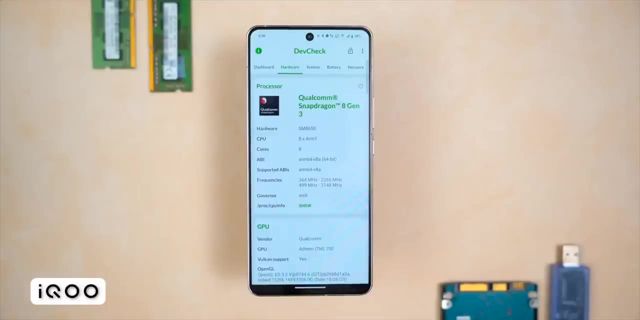 Coming to iQOO, I would say they did a really good work. in 2023. They launched a few phones: iQOO Neo 7, iQOO Neo 7 Pro and, just recently, the iQOO 12,, which is the first phone in India with Snapdragon 8 Gen 3.. 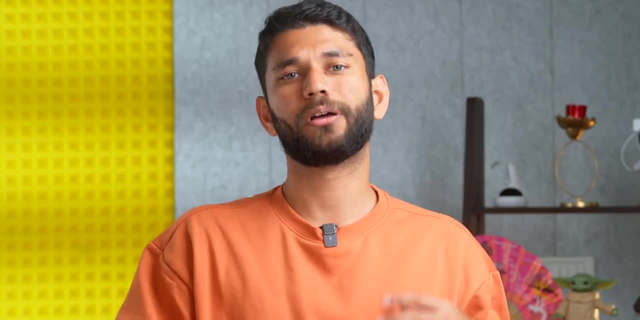 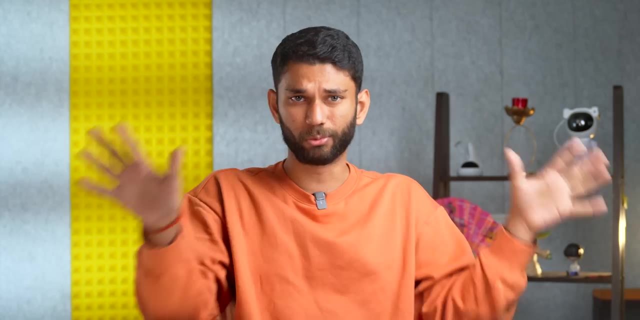 iQOO has this trend of giving great performance at a reasonable price. Now, yes, to give superior performance on a budget, iQOO has to make compromises. Like the iQOO Neo 7 didn't have an ultra-wide angle camera, which is totally understandable. 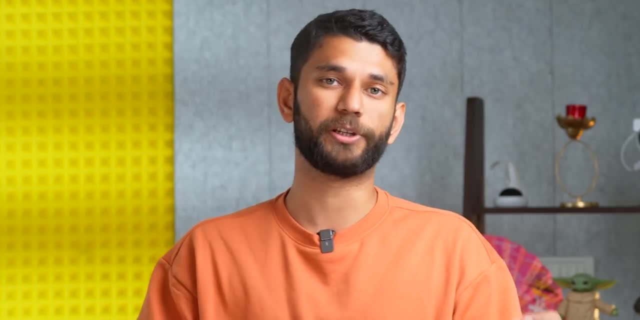 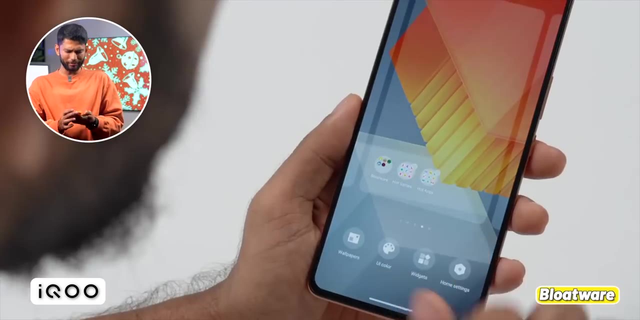 That being said, the only concern I have with iQOO phones is the software experience. Like the software has improved over time, iQOO 12 has no hot apps or hot games, but there are still occasional bloatwares and few ads. 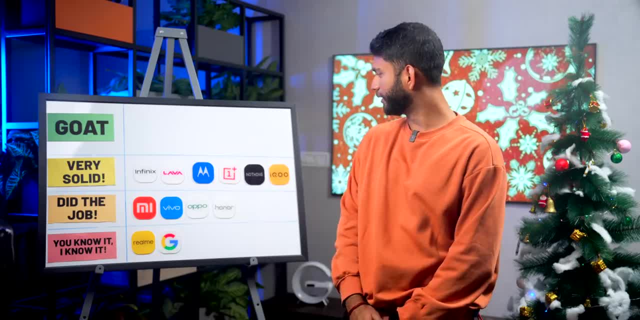 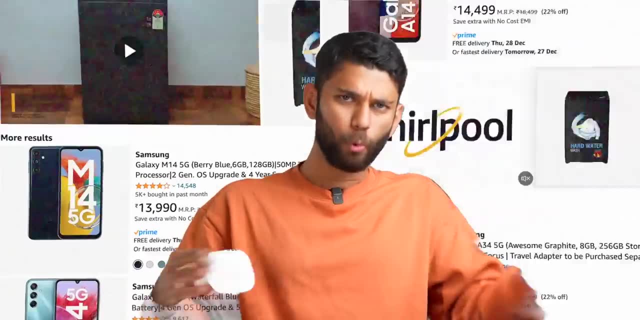 So I'll put iQOO in very solid tier. And finally we have Samsung, which is the most interesting brand Now. I say interesting because, A- Samsung has so many phones- like they have more than one phone in every price bracket- And, B- the experience of using these phones are very different. 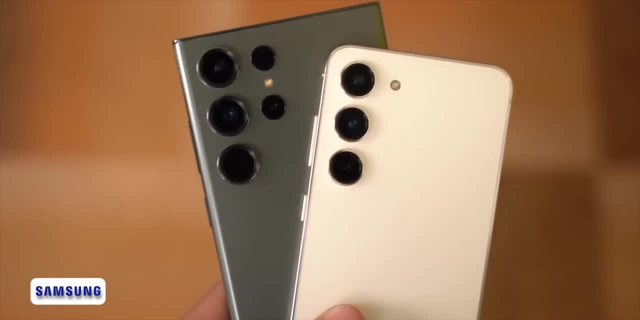 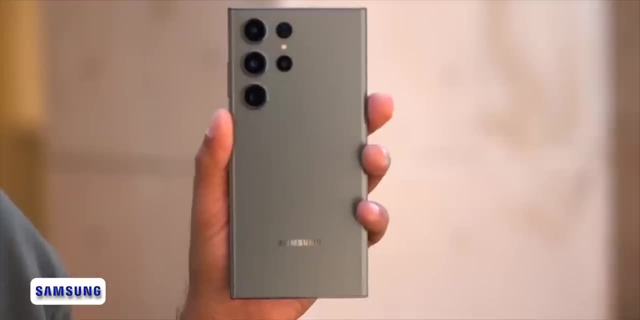 Like on one end. we have premium and flagship phones like the S23 series, the FE series, Z Fold and Z Flip, and even A series like the A54 and A34.. All these phones have awesome display, great camera and probably the best. 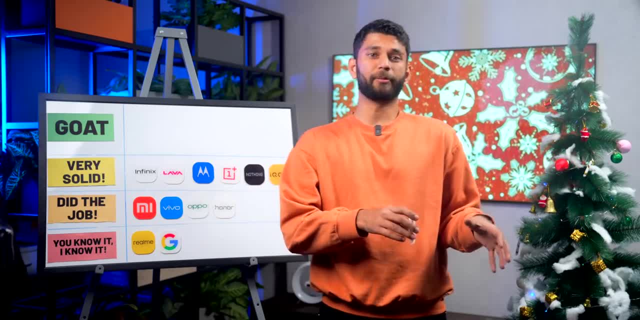 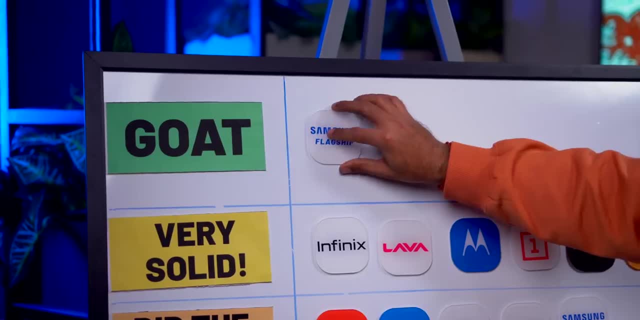 Android software experience that we see. Plus, Samsung promises 4 years of software updates and 5 years of security patches, which they are delivering really well. So these Samsung flagship phone goes into goat tier, But also, on the other hand, Samsung also launches budget phones like the FNM series. 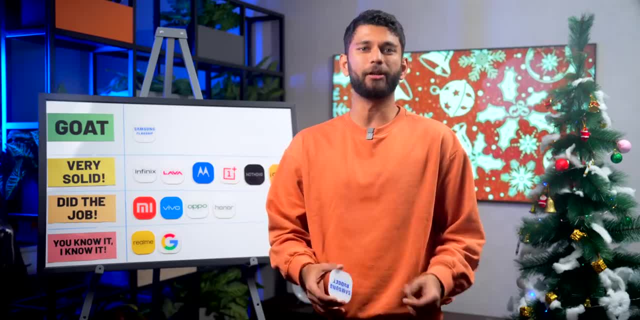 The story here is completely opposite. I mean, they are average phones at best and do not have good value for money. Plus, the software is like a cut down version of the main one UI, So you don't get features, you get a lot of features. 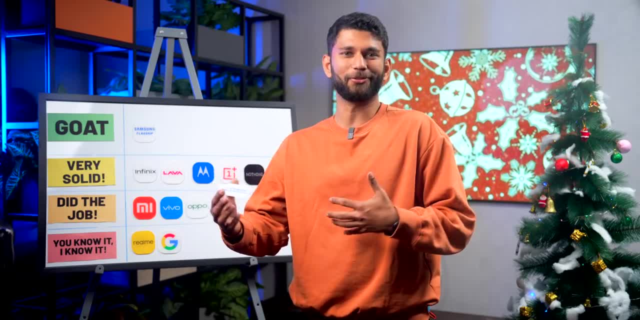 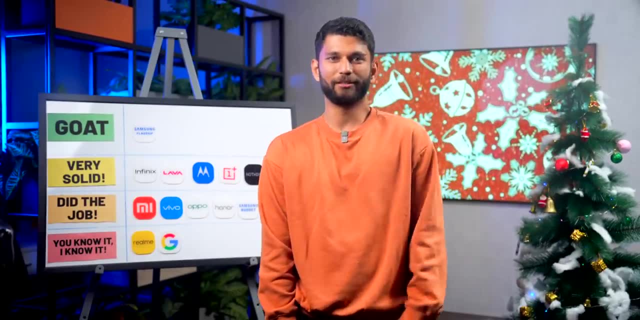 Like secure folder and all of that. It seems as if Samsung has a lot of children. Only a few of them get the best treatment, So the Samsung budget goes into did the job tier. Indian parents will relate to this. That's a very dark joke. 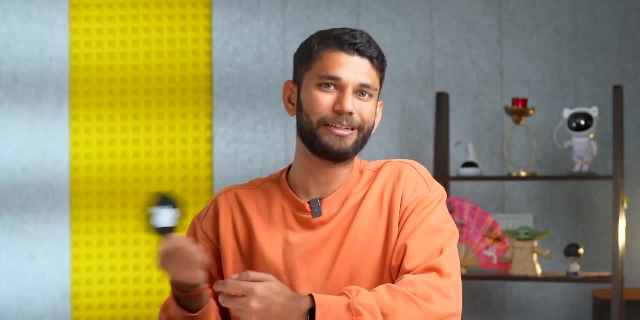 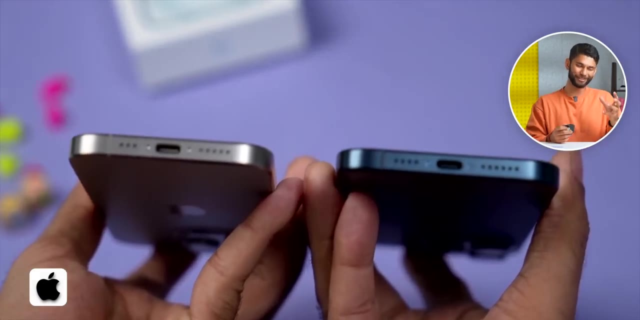 Other things that Indian will relate to is brand value, And in that respect, Apple tops the chart. Now, 2023 was one of the most happening years for Apple. Firstly, they were forced to make the iPhone 15 type C. Thank you, EU. 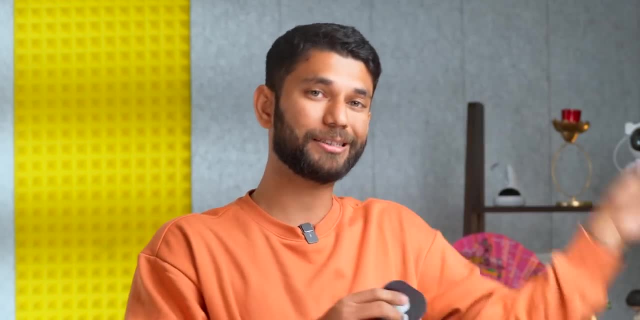 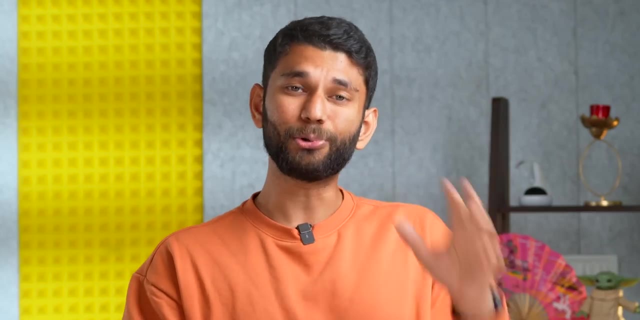 Second, all the innovation that we saw with the expensive iPhone 14 Pro of last year made its way to the left. And third, they really pushed the boundaries this year with cameras, Like when we compared them against the Samsung and Google, 8 out of 10 times iPhone's photo were the better ones.